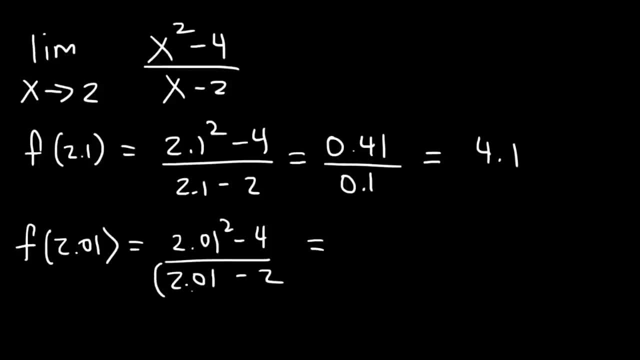 So if you type this in the way you see it in your calculator, you may have to put this in parentheses. You should get 4.01.. So notice what's happening: As we get closer and closer to 2, the limit approaches 4.. So we could therefore say that the limit as x approaches 2 of this function. 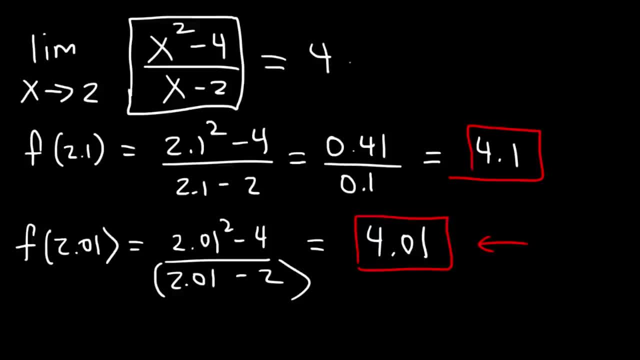 is equal to 4.. And this technique works for any limit, As long as you plug in a number that's very close to whatever this number is, but not exactly that number. if the limit exists, it's going to converge to a certain value. 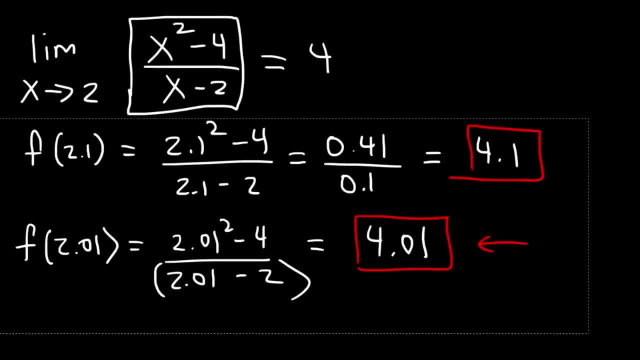 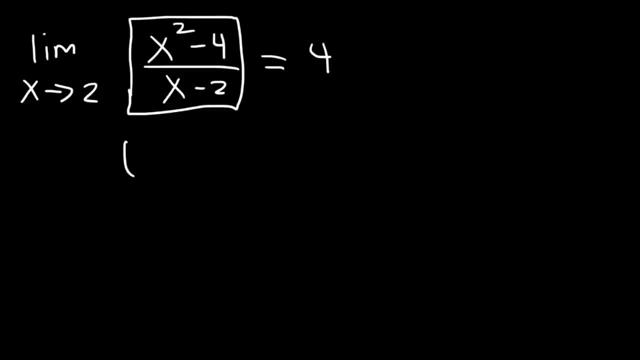 Now sometimes you have to use other techniques to get the answer. In this particular example, we could factor x squared minus 4, you can write it as x plus 2 times x minus 2.. Now we need to rewrite the limit expression until we replace x with 2.. 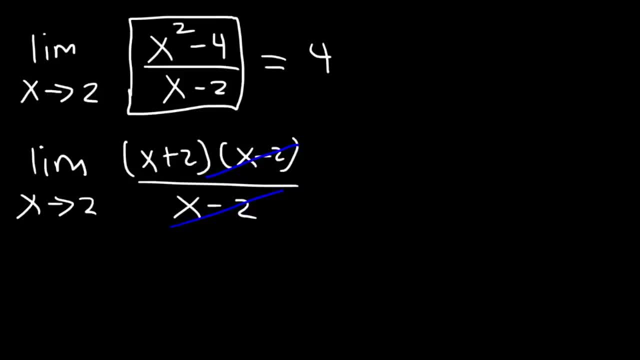 Now notice that we can cancel x minus 2.. So when this term is gone, we can now use direct substitution, because the x minus 2 factor was given us a 0 in the denominator, which we don't want. So now all we need to do is find the limit, as x approaches 2, of x plus 2.. 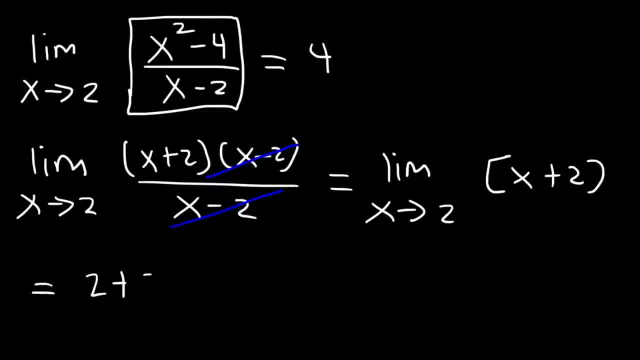 So now we can replace x with 2,, and 2 plus 2 is 4.. And so that's the limit: It approaches a value of 4.. Now let's look at another example. What is the limit as x approaches 2?? 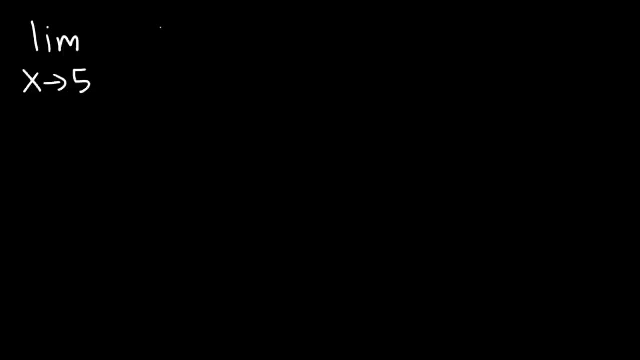 limit as x approaches, 5 of x squared plus 2x minus 4.. So notice that we don't have a fraction. We're not going to get a 0 in a denominator, So for a question like this you can use direct substitution. So all you got to do is plug in 5.. So it's going to be. 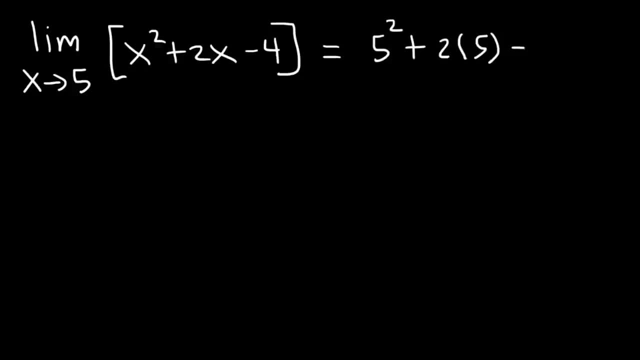 5 squared plus 2 times 5 minus 4.. So that's 25 plus 10 minus 4, and 25 plus 10 is 35. So the limit is going to be 31.. And so that's it for that example. But now what about this? 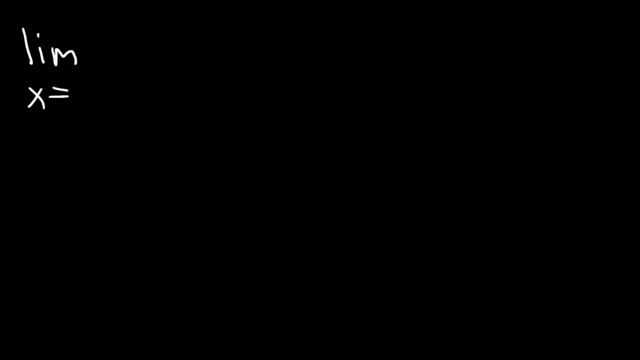 one. What is the limit, as x approaches 3, of x cubed minus 27 over x minus 3?? Now if we try to plug in 3, it's going to be 0 over 0. So we don't want to do that In this case. 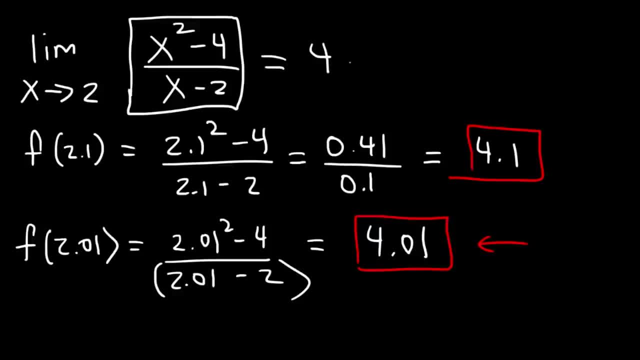 is equal to 4.. And this technique works for any limit, As long as you plug in a number that's very close to whatever this number is, but not exactly that number. if the limit exists, it's going to converge to a certain value. 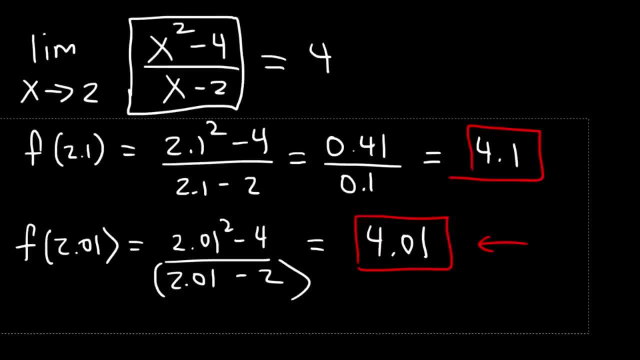 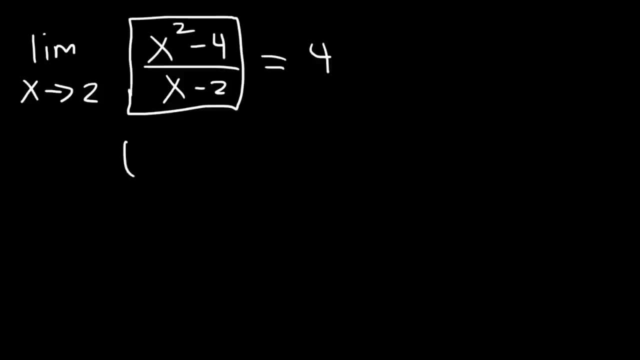 Now sometimes you have to use other techniques to get the answer. In this particular example, we could factor x squared minus 4, you can write it as x plus 2 times x minus 2.. Now we need to rewrite the limit expression until we replace x with 2.. 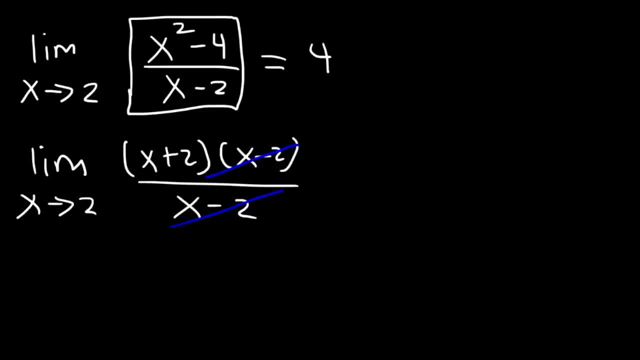 Now notice that we can cancel x minus 2.. So when this term is gone, we can now use direct substitution, because the x minus 2 factor was given us a 0 in the denominator, which we don't want. So now all we need to do is find the limit, as x approaches 2, of x plus 2.. 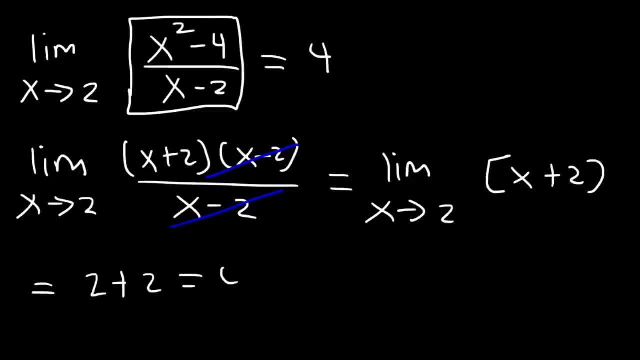 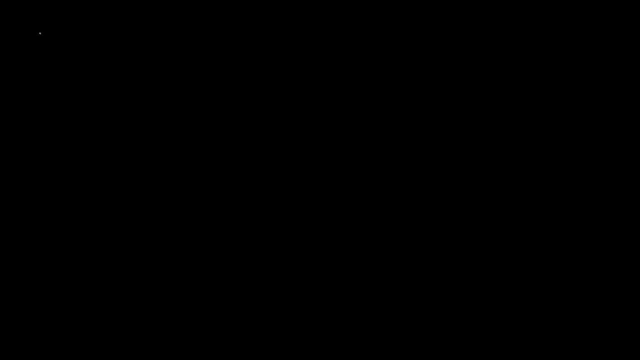 So now we can replace x with 2, and 2 plus 2 is 4.. And so that's the limit: It approaches a value of 4.. Now let's look at another example. What is the limit? What is the limit as x approaches 5 of x squared plus 2x minus 4?? 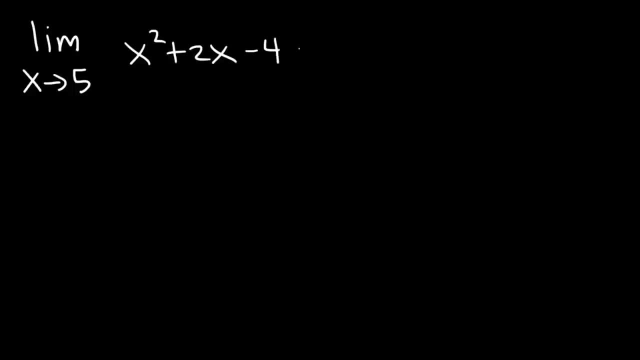 So notice that we don't have a fraction. We're not going to get a 0 in the denominator, So for a question like this you can use direct substitution. So all you got to do is plug in 5.. So it's going to be 5 squared plus 2 times 5 minus 4.. 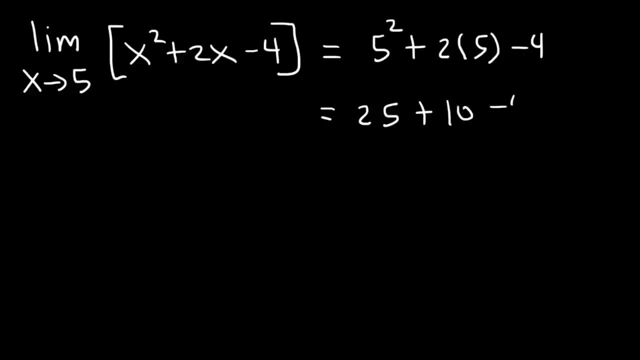 So that's 25 plus 10.. Minus 4 and 25 plus 10 is 35. So the limit is going to be 31.. And so that's it for that example. But now what about this one? What is the limit as? 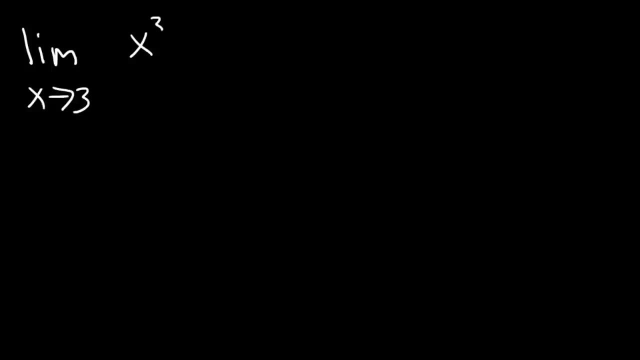 x approaches 3 of x cubed minus 27 over x minus 3? Now if we try to plug in 3, it's going to be 0 over 0. So we don't want to do that In this case. 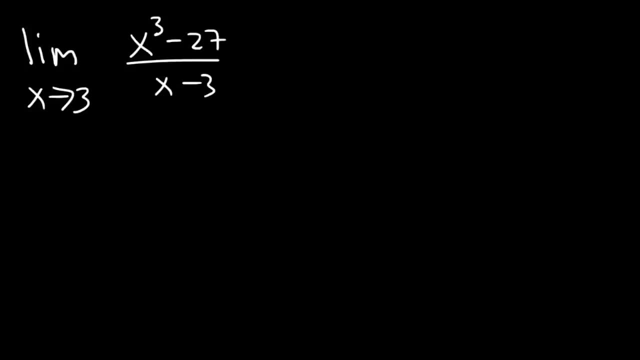 if you have a fraction like this, see if you can factor the expression. So how can we factor x cubed minus 27?? So what we have is the difference of cubes. And whenever you see that you can use this formula, a cubed minus b cubed is. 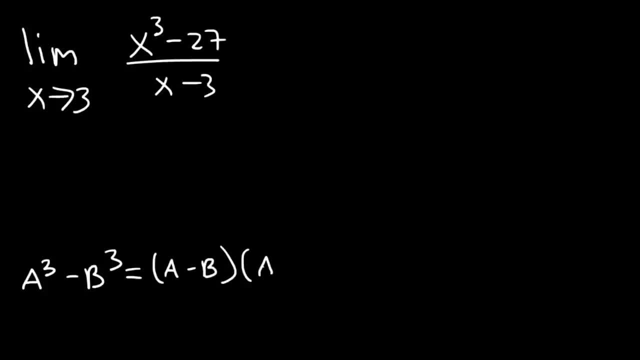 a minus b times a squared plus a, b plus b squared. So in our example a to the third is like x to the third and b to the third is 27.. So a is the cube root of x cubed, which is x. 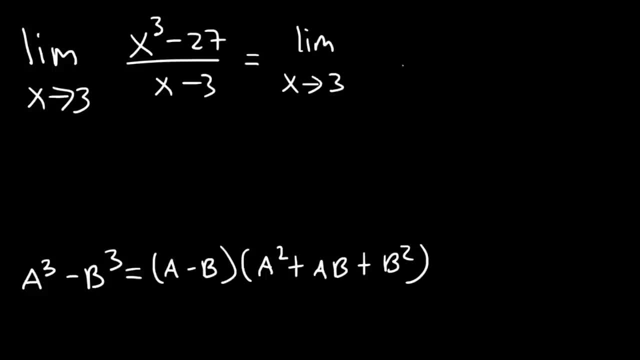 So a is the cube root of x, cubed, which is x, And b is the cube root of 27,, which is 3.. So this is going to be x minus 3, and then a squared, That's x squared, And then plus a, b, So that's 3 times x and then plus b squared, or 3 squared, which is 9.. 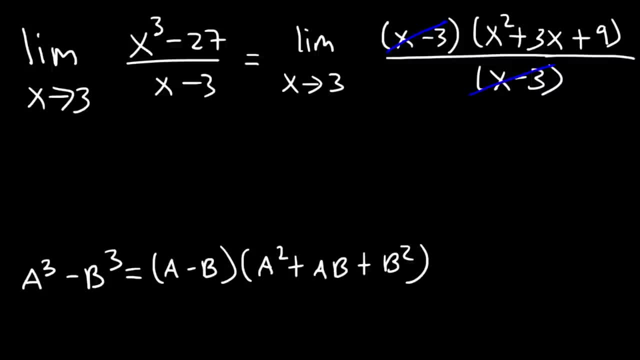 So now we can cancel the factor x minus 3.. So what we have left over is the limit, as x approaches 3, of x squared plus 3x plus 9.. So at this point we now can use direct substitution. So it's 3 squared plus 3 times 3. 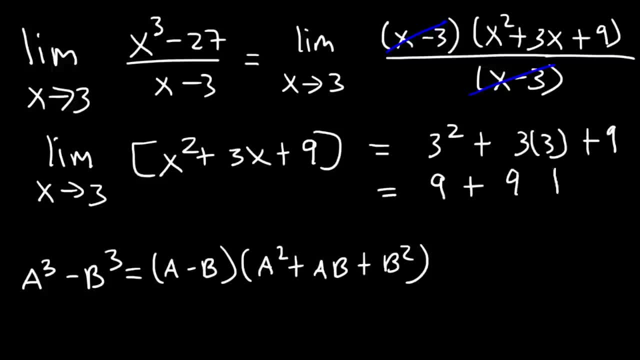 plus 9,, which is 9 plus 9 plus 9.. Adding 9 three times is basically multiplying 9 by 3. And so this limit is equal to 27.. Now here's another problem that you can work on. 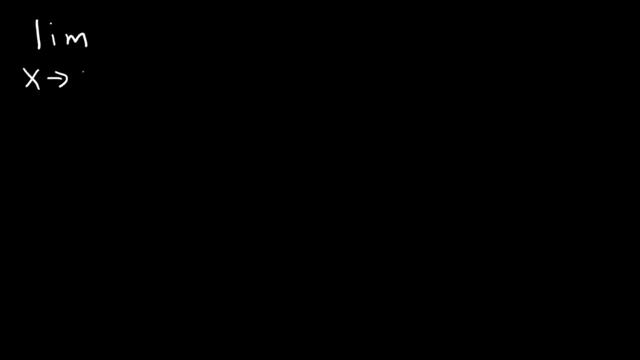 So what is the limit, as x approaches 3, of 1 over x minus 1 over 3 divided by x minus 3?? So for these examples, feel free to pause the video if you want to and try these problems. So in this example we have a complex fraction. 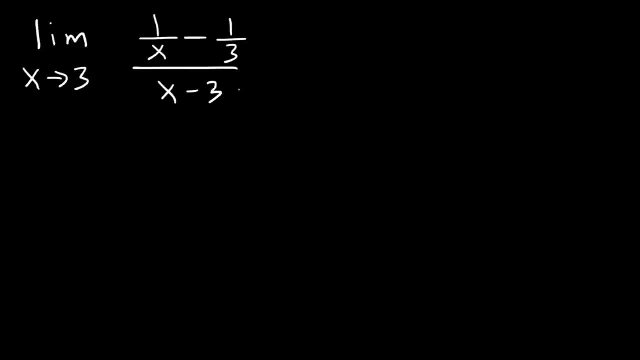 So what do you do in a situation like this, If you get a complex fraction? what I recommend is to multiply the top and the bottom by the common denominator of those two fractions, That is, by x and by 3.. So I'm going to multiply the top and the bottom by 3x. 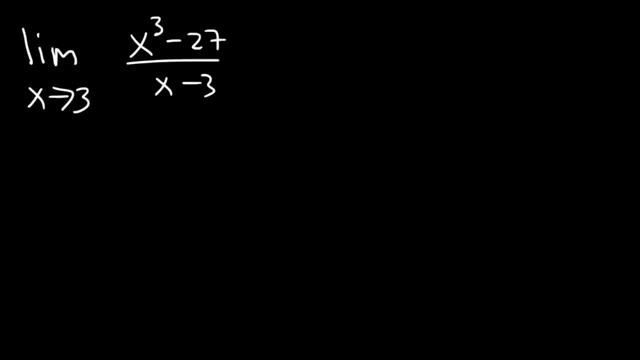 if you have a fraction like this, see if you can factor the expression. So how can we factor x cubed minus 27?? So what we have is the difference of cubes. And whenever you see that you can use this formula: a cubed minus b cubed is a minus b times a squared plus a b. 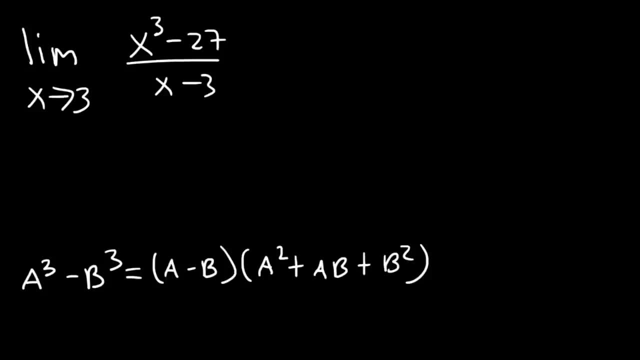 plus b squared, So that's a squared minus b squared, So that's a squared minus b squared. So in our example, a to the third is like x to the third and b to the third is 27.. So a is the cube root of x cubed, which is x, And b is the cube root of 27,, which is 3.. So this is going to. 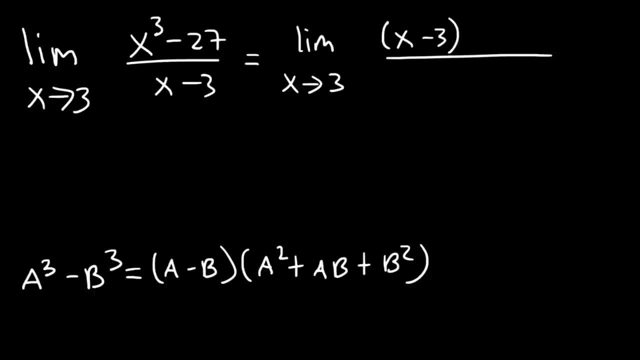 be x minus 3 and then a squared, that's x squared, and then plus ab, So that's 3 times x and then plus b squared, or 3 squared, which is 9.. So now we can cancel the factor x minus 3.. 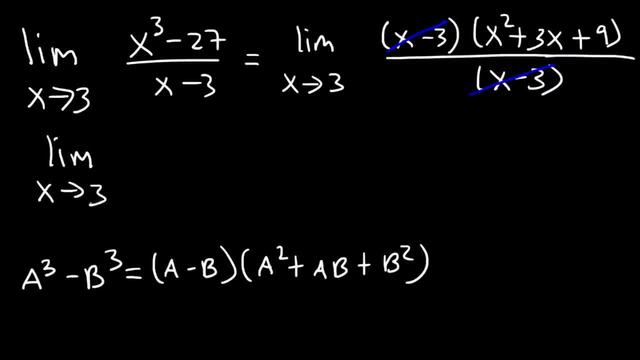 So what we have left over is the limit as x approaches, 3 of x squared plus 3x plus 9.. So at this point we now can use direct substitution. So it's 3 squared plus 3 times 3 plus 9, which is 9 plus 9 plus 9.. 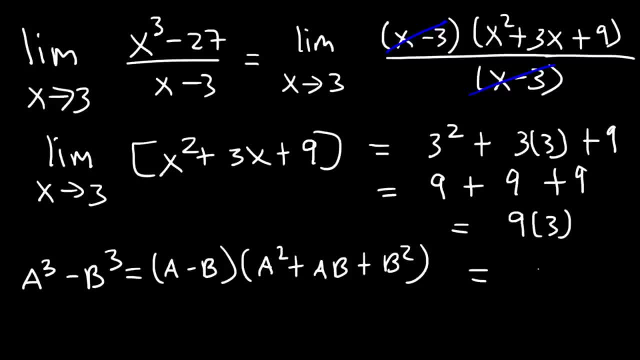 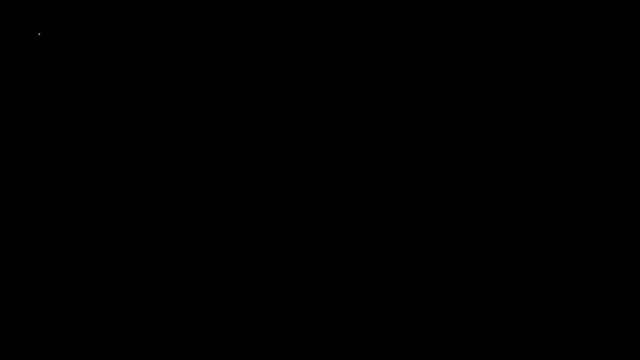 Adding 9 three times is basically multiplying 9 by 3.. And so this limit is equal to 27.. Now here's another problem that you can work on. So what is the limit, as x approaches 3, of 1 over x minus 1 over 3?? 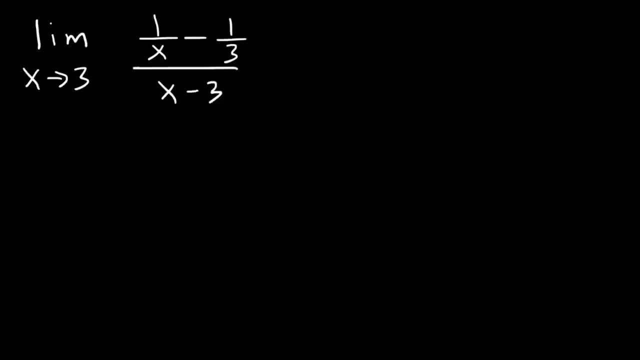 3 divided by x minus 3.. So for these examples, feel free to pause the video if you want to and try these problems. So in this example we have a complex fraction. So what do you do in a situation like this? 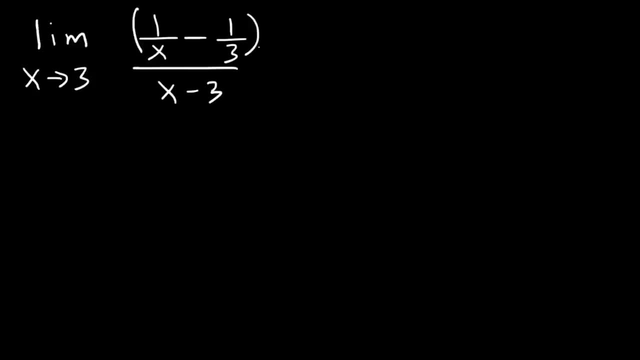 If you get a complex fraction, what I recommend is to multiply the top and the bottom by the common denominator of those two fractions, That is, by x and by 3.. So I'm going to multiply the top and the bottom by 3x. 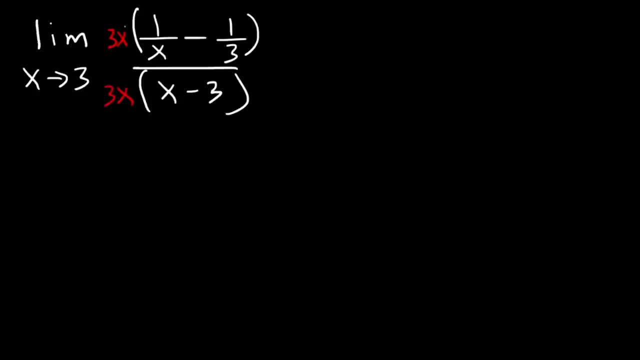 So if we multiply 3x by 1 over x, the x variables will cancel, And so what we're going to have left over is simply 3.. And if we multiply 3x by 1 over 3, the 3's will cancel, leaving behind x. but there's. 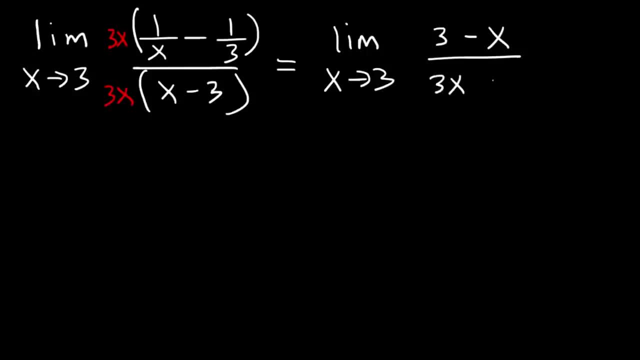 a negative sign in front of it. Now for the terms on the bottom. I'm going to leave it in its factored form. So notice that 3 minus x and x minus 3 are the same. If you see a situation like this, factor out a negative 1.. 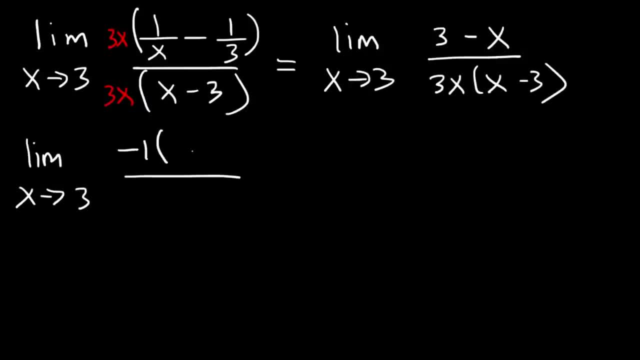 If we take out a negative 1, the negative x will change to positive x And positive 3 will change to negative 3.. So notice that we can cancel the x minus 3 factor at this point, And so what we have left over is the limit. 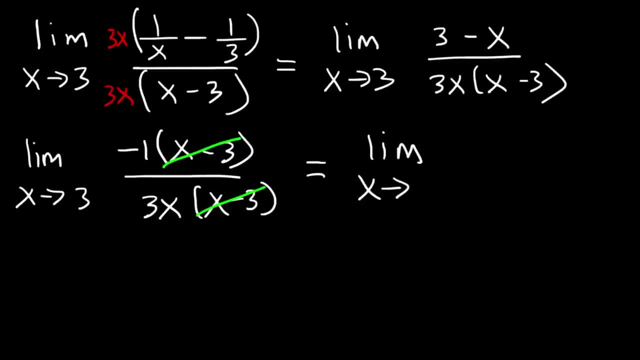 And so what we have left over is the limit, And so what we have left over is the limit, and so on. that, as x approaches 3 of negative 1 over 3x, So now we can use direct substitution. So let's replace x with 3.. 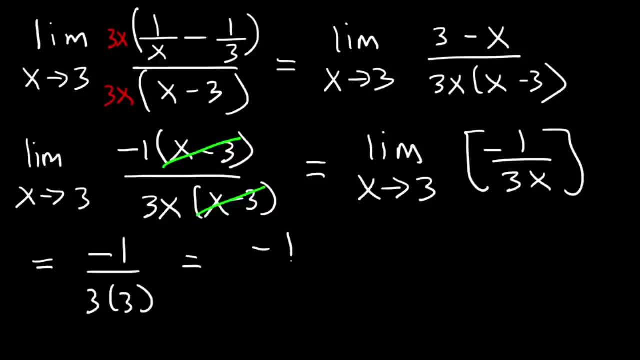 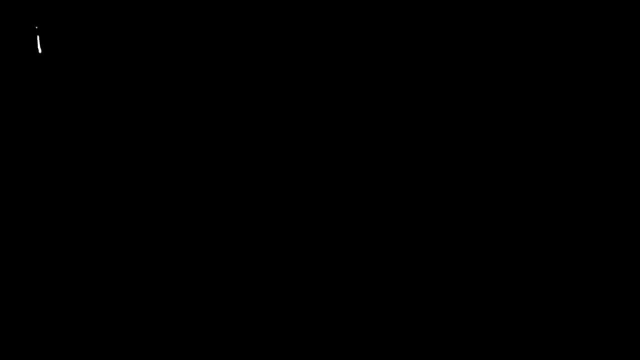 So it's going to be 3 times 3, which is none, not. so the final answer is negative: 1 divided by 9.. So now you know how to evaluate limits that are associated with complex fractions. So here's another example: What is the limit, as x approaches 9, of square root x minus 3 over x minus 9?? 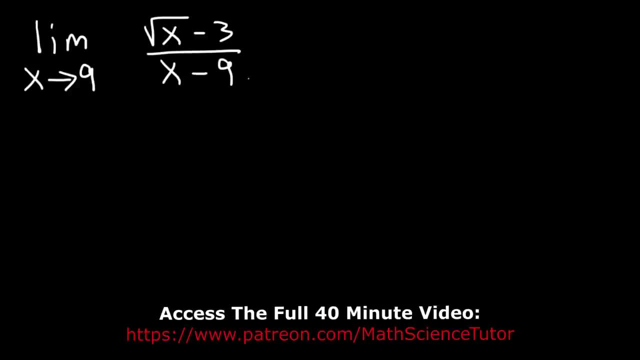 So what should we do if we're dealing with square roots? What I recommend is to multiply the top and the bottom by the conjugate of the expression that has a square root. So the conjugate of square root x minus 3 is square root x plus 3.. 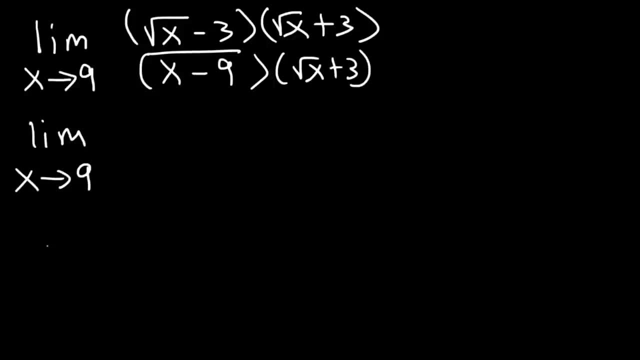 So in the numerator we need to FOIL: So the square root of x times the square root of x is the square root of x squared, which is simply x, And then we have the square root of x times 3, so that's going to be plus 3 square root x. 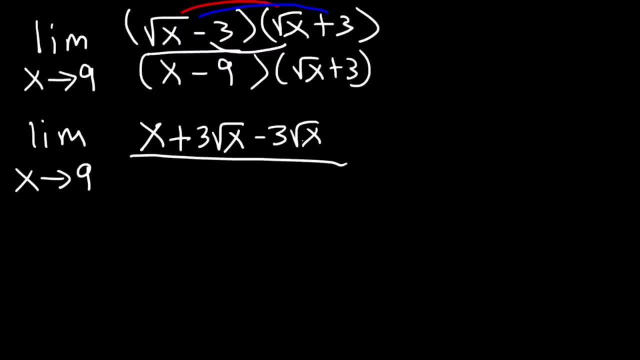 and then these two will form negative 3, square root x, And finally we have negative 3 times positive 3, which is negative 9.. Now on the bottom. I'm going to multiply the top and the bottom by the conjugate of x. 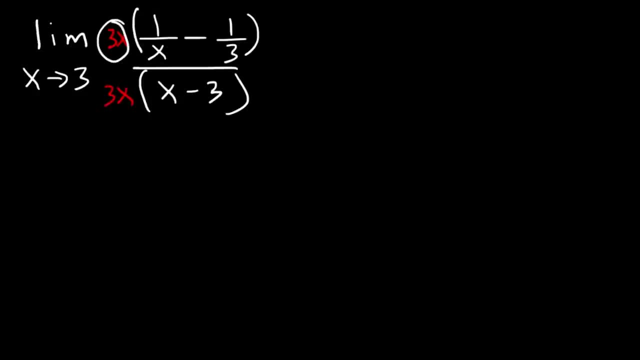 So if we multiply 3x by 1 over x, the x variables will cancel, And so what we're going to have left over is simply 3.. And if we multiply 3x by 1 over 3,, the 3s will cancel. 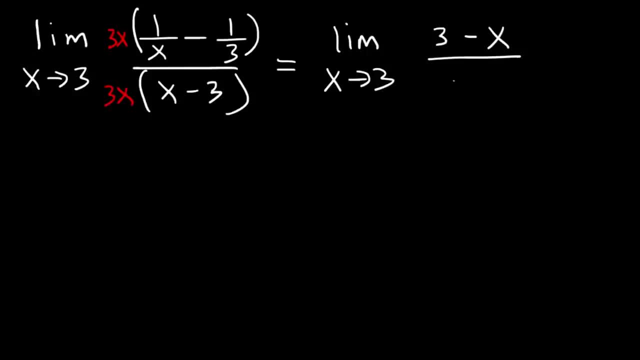 leaving behind x, but there's a negative sign in front of it. Now for the terms on the bottom. I'm going to leave it in its factored form. So notice that 3 minus x and x minus 3 are very similar. 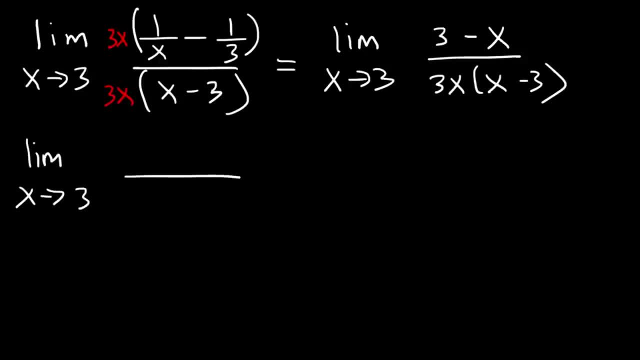 If you see a situation like this, factor out a negative 1.. If we take out a negative 1, the negative x will change to positive x And positive 3, will change to negative 3.. So notice that we can cancel the x minus 3 factor at this point. 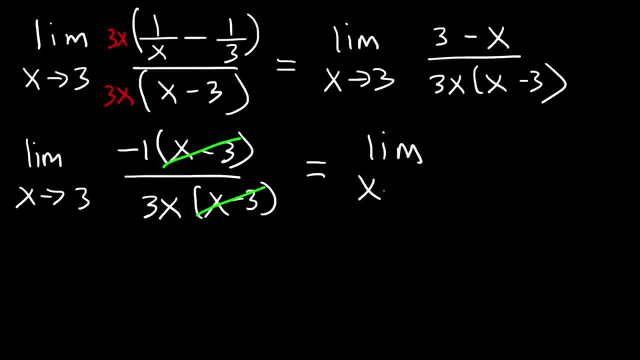 And so what we have left over is the limit, as x approaches 3, of negative 1 over 3x. So now we can use direct substitution. So let's replace x with 3.. So it's going to be 3 times 3,. 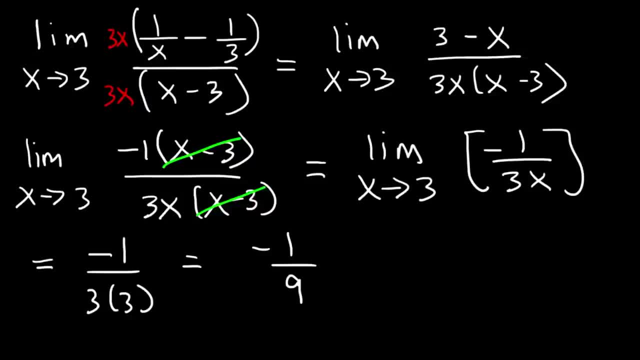 which is 9.. So the final answer is negative: 1 over 3x. So the final answer is negative: 1 over 3x. So now you know how to evaluate limits that are associated with complex fractions. So here's another example. 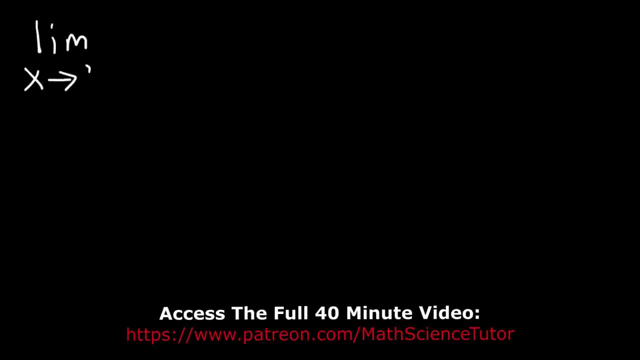 What is the limit, as x approaches 9, of square root x minus 3 over x minus 9?? So what should we do if we're dealing with square roots? What I recommend is to multiply the top and the bottom by the conjugate of the expression that has a square root. 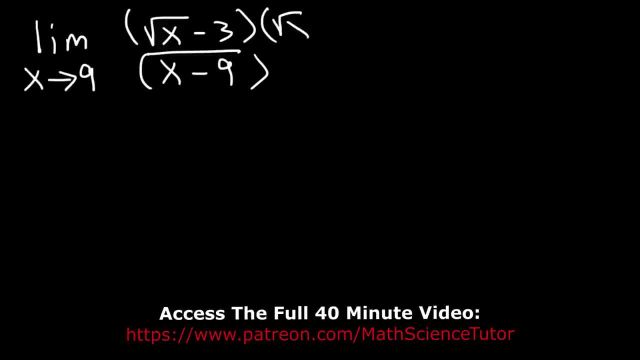 So the conjugate of square root x minus 3 is square root x plus 3.. So in the numerator we need to FOIL: So the square root of x times the square root of x is the square root of x squared, which is simply x. 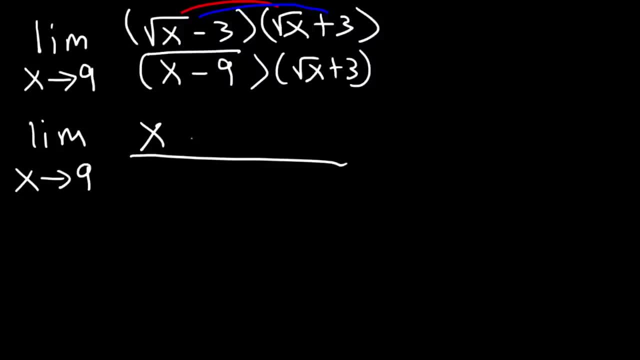 And then we have the square root of x times 3.. So that's going to be plus 3 square root x, And then these two will form negative 3 square root x And finally we have negative 3 times positive 3,. 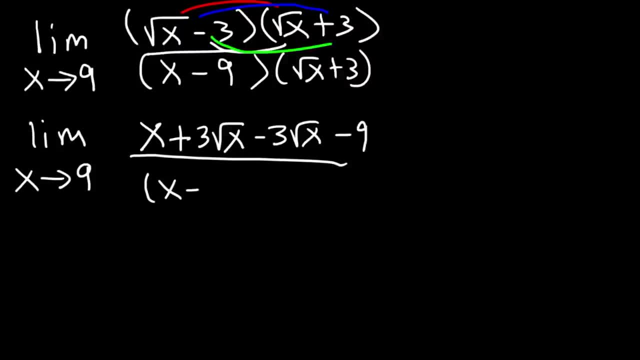 which is negative 9.. Now on the bottom, I'm not going to FOIL the two expressions, I'm going to leave it the way it is, because my goal is to get rid of the x minus 9.. I want to cancel it. 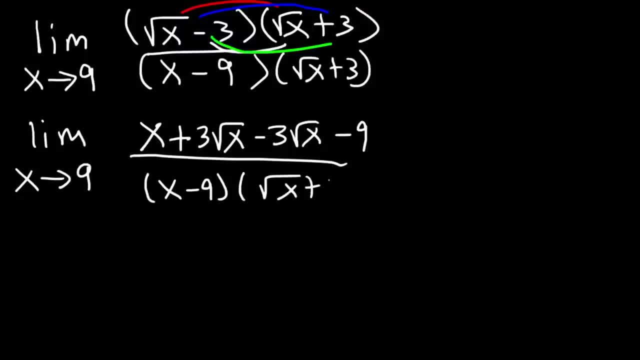 But I'm not going to FOIL the two expressions. I'm going to leave it the way it is, Because my goal is to get rid of the x minus 9.. I want to cancel it. So now: negative 3 and positive 3 add up to 0. 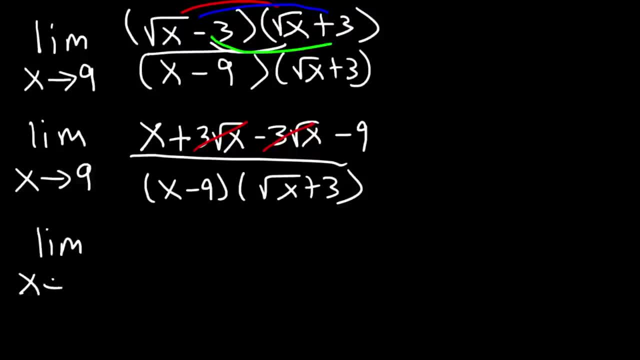 So what we have left over is the limit, as x approaches 9, of x minus 9 divided by x minus 9 times the square root of x plus 3.. So now, at this point, notice that we can cancel x minus 9.. 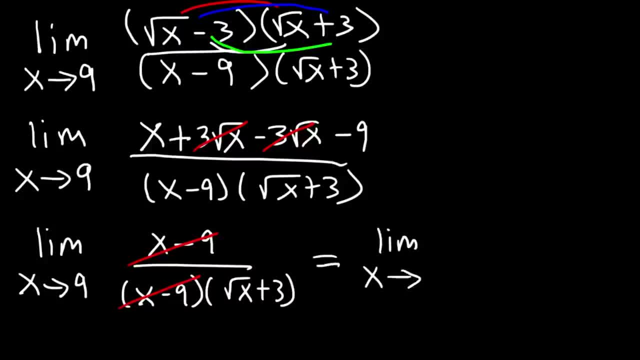 And so what we have is a square root of x plus 3.. So what we have left over is the limit, as x approaches 9, of 1 over square root x plus 3.. So now what we can do is replace x with 9.. 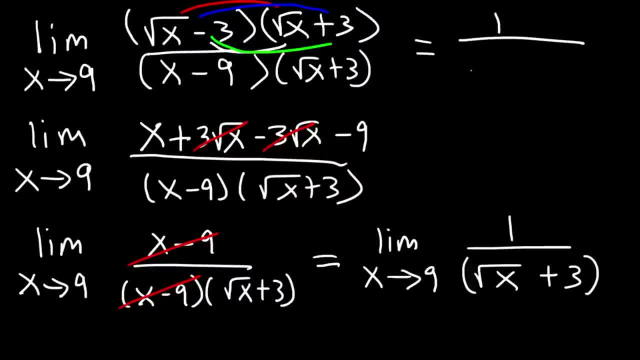 So I'm just going to continue up here. So it's going to be 1 over square root 9 plus 3.. And the square root of 9 is 3.. And 3 plus 3 is 6.. So the final answer is 1 over 6.. 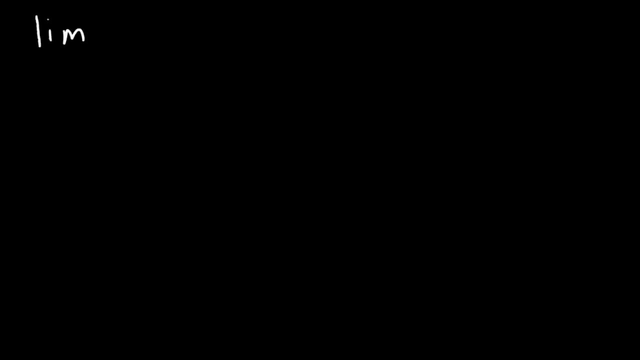 Now let's look at this example. What is the limit, as x approaches 4, of the expression 1 over square root, x minus 1 over 2 divided by x minus 4?? So this time we have a complex fraction with radicals. 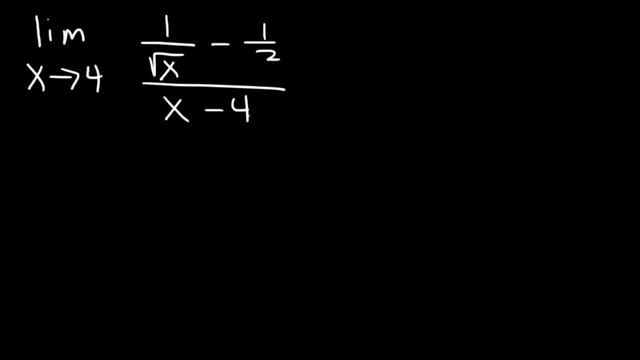 That means we need to multiply the top and the bottom not only by the common denominator but also by the conjugate. But let's start with the common denominator. So I'm going to multiply the top and the bottom by these two, That is, by 2 square root x. 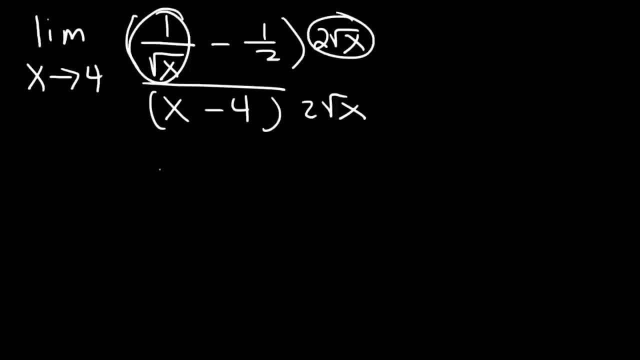 So when I multiply 1 over square root x times 2, square root x, the square root x terms will cancel, leaving behind positive 2.. So I have the limit as x approaches 4 with a 2 on top, And if I multiply these two, 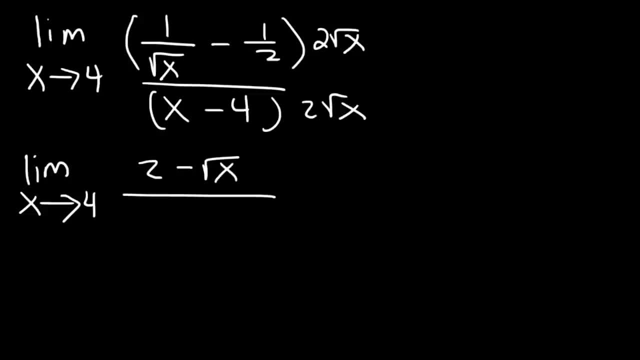 the 2's will cancel, leaving behind the square root of x. And so on the bottom, I have 2 square root x times x minus 4.. So now my next step is to multiply the top and the bottom by the conjugate of the radical expression. 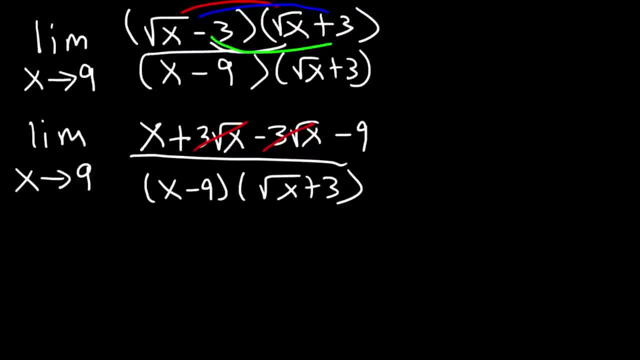 So now negative 3 and positive 3 add up to 0.. So what we have left over is the limit, as x approaches 9, of x minus 9 divided by x minus 9 times the square root of x plus 3.. So now, at this point, 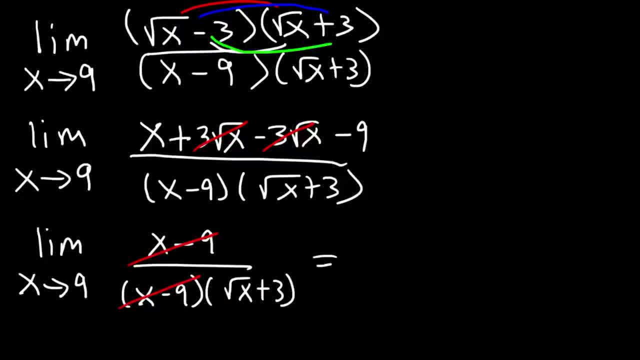 notice that we can cancel x minus 9.. And so what we have left over is the limit, as x approaches 9, of 1 over square root x plus 3.. So now what we can do is replace x with 9.. So I'm just going to. 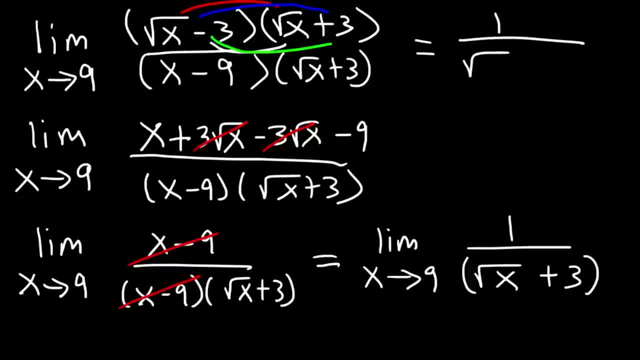 I'm going to continue up here. So it's going to be 1 over square root, 9 plus 3.. And the square root of 9 is 3. And 3 plus 3 is 6.. So the final answer is 1 over 6.. 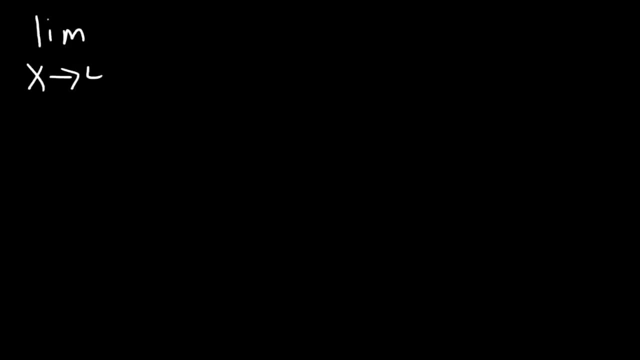 Now let's look at this example. What is the limit, as x approaches 4, of the expression 1 over square root? x minus 1 over 2? E Divided by x minus 4.. So this time we have a complex fraction with radicals. 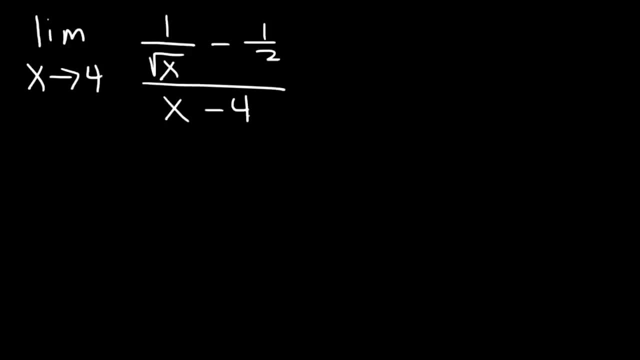 That means we need to multiply the top and the bottom not only by the common denominator but also by the conjugate. But let's start with the common denominator. So I'm going to multiply the top and the bottom by these two, That is, by 2 square root x. 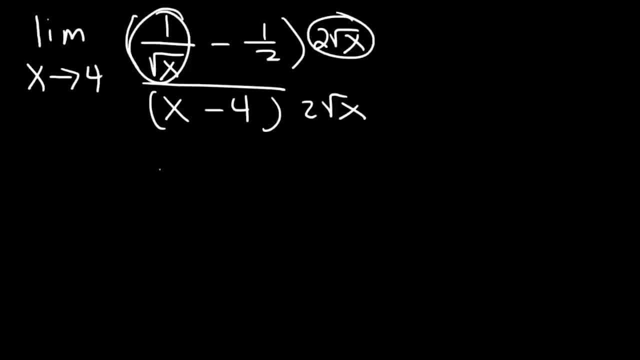 So when I multiply 1 over square root x times 2 square root x, the square root x terms will cancel, leaving behind positive 2.. So I have the limit as x approaches 4 with a 2 on top And if I multiply these two, the 2s will cancel, leaving behind the square root of x. 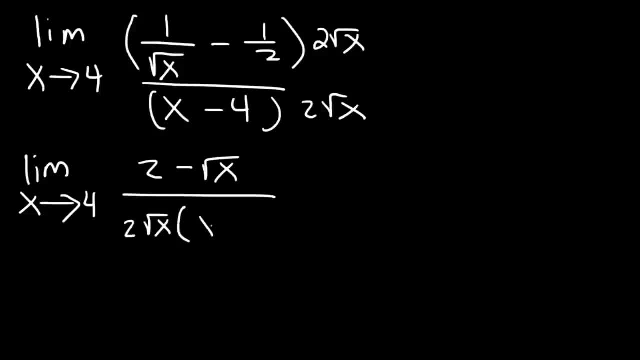 And so on the bottom I have 2 square root x times x minus 4.. So now my next step is to multiply the top and the bottom by the conjugate of the radical expression, that is, by 2 plus square root x. 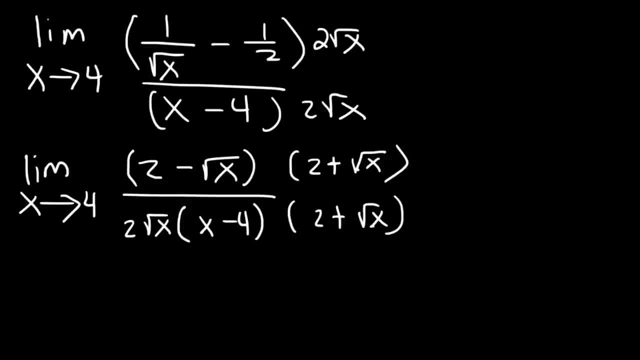 Now I'm only going to FOIL the top part, not the bottom. So we have 2 times 2, which is 4.. And then we have 2 times the square root of x, And then these two, that's going to be negative 2 square root x. 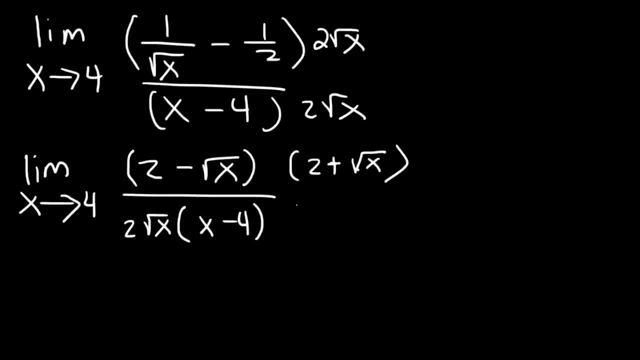 That is by 2 plus square root x. Now I'm only going to FOIL the top part, not the bottom. So we have 2 times 2, which is 4.. And I'm going to FOIL the top part, not the bottom. 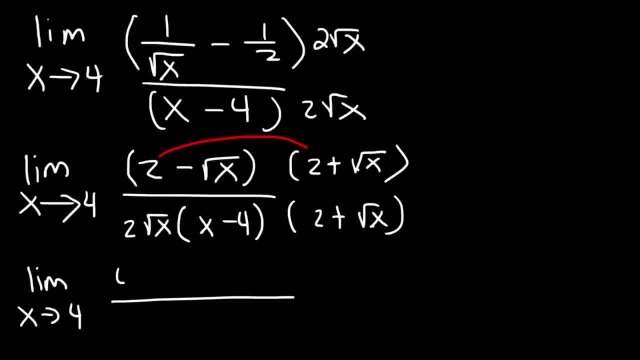 So we have 2 times 2,, which is 4.. And I'm going to FOIL the top part, not the bottom. So we have 2 times 2,, which is 4.. And then we have 2 times the square root of x. 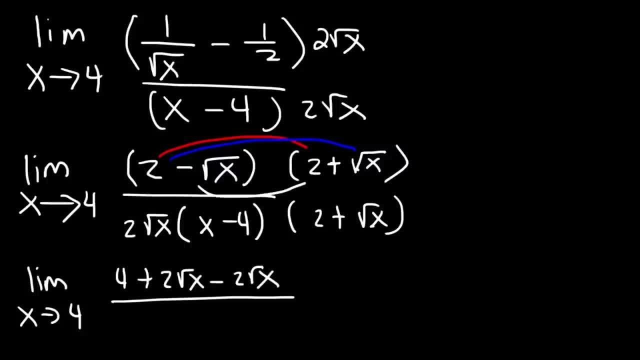 And then these two, that's going to be negative 2 square root x And negative square root x times positive square root x is going to be negative square root x squared, which is negative x. And in the denominator don't FOIL. 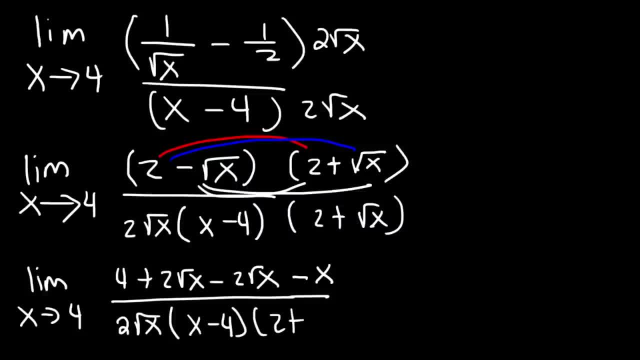 Just rewrite what you have. If you follow these steps won't be that difficult. So now, 2 and negative 2 adds up to 0. So what we have left over is the limit, as x approaches 4, of 4 minus x divided by all the stuff. 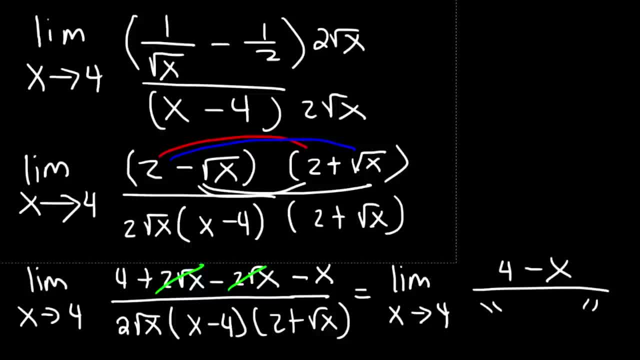 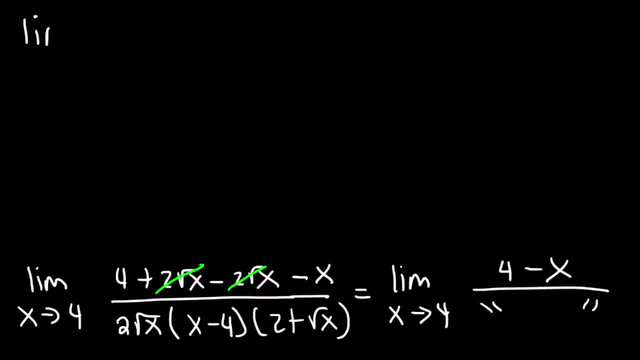 that we have on the bottom. Now, what we're going to do at this point is we're going to factor out a negative 1.. So this is now the limit as x approaches 4.. So negative 1, and this is going to change to positive x and plus 4 is going to. 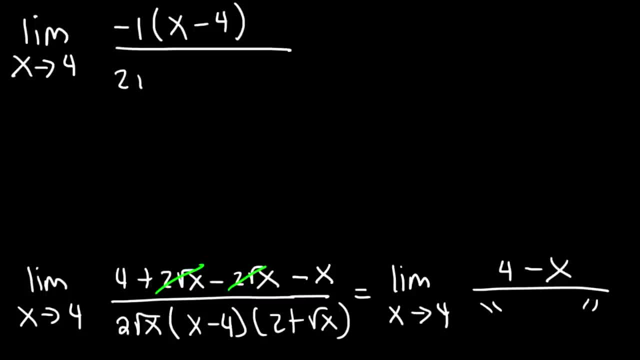 change to negative 4, just like we did before. So now notice that we can cancel the x plus 4 terms at this point. So this is what we have left over. So now let's replace x with 4.. So it's negative 1 divided by 2 square root 4. 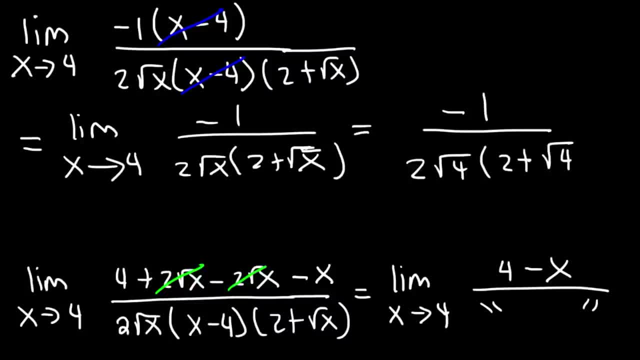 times 2 plus square root 4.. So the square root of 4 is 2, and 2 times 2, that's going to be 4, and 2 plus 2 is 4.. And 4 times 4 is 16.. So the final answer is negative: 1 divided by 16.. And so that's. 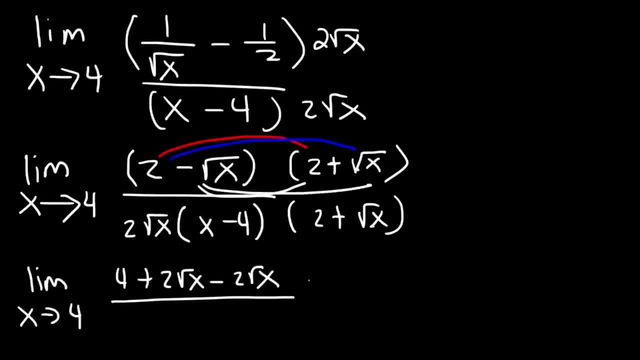 And negative square root x times positive. So negative square root x is going to be negative square root x squared, which is negative x. And in the denominator don't FOIL, just rewrite what you have. If you follow these steps, it won't be that difficult. 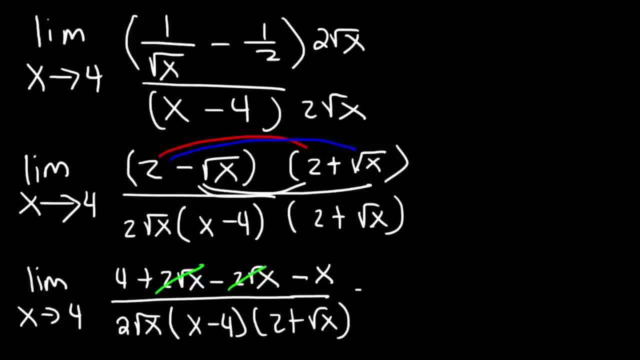 So now, 2 and negative 2 adds up to 0. So what we have left over is the limit as x approaches, 4 of 4 minus x divided by all the stuff that we have left over. So that's the limit, So that's the limit. 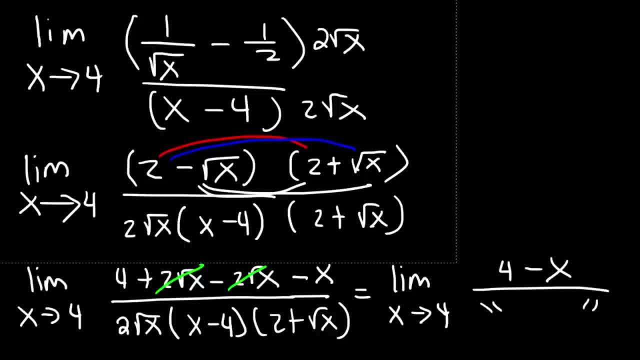 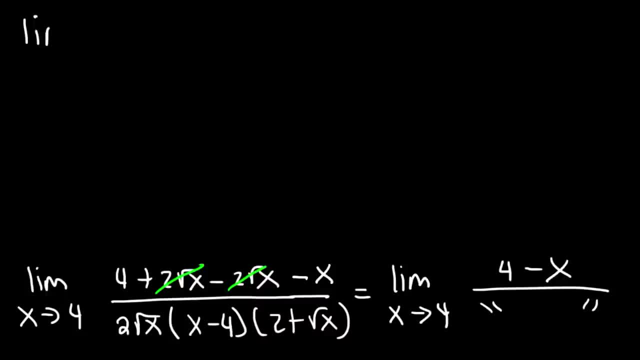 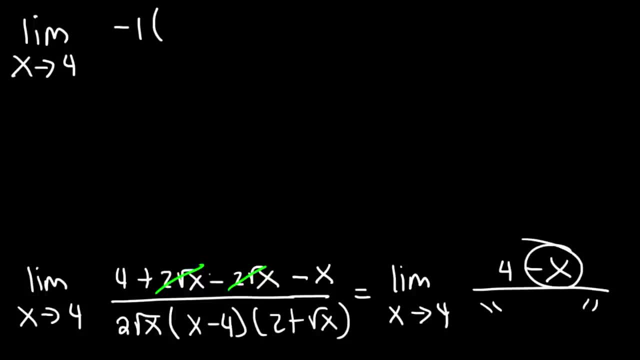 So negative 1. And this is going to change to positive x And plus 4 is going to change to negative 4.. Just like we did before, So now notice that we can cancel the x plus 4 thing. So now we have 4 terms at this point. 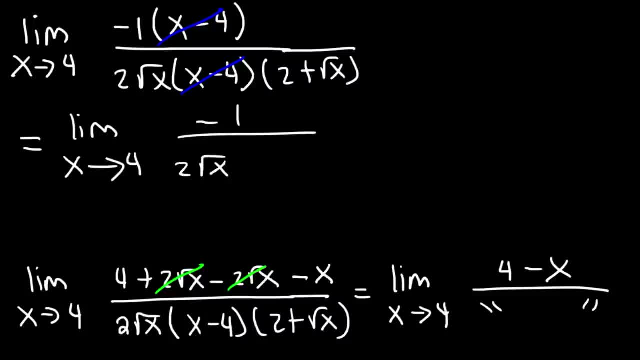 So this is what we have left over. So now let's replace x with 4.. So it's negative 1 divided by 2, square root 4 times 2 plus 4.. Square root 4.. So the square root of 4 is 2.. 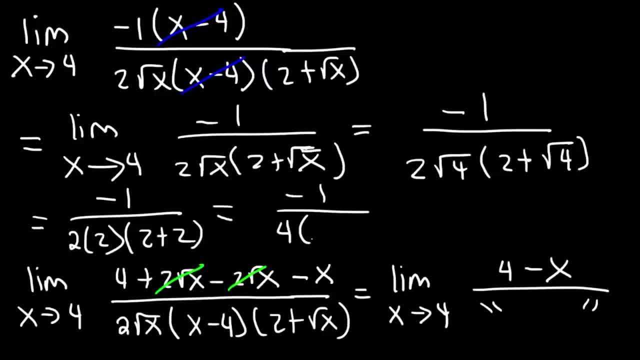 And 2 times 2,, that's going to be 4.. And 2 plus 2 is 4.. And 4 times 4 is 16.. So the final answer is negative 1 divided by 16., And so that's going to be the limit. 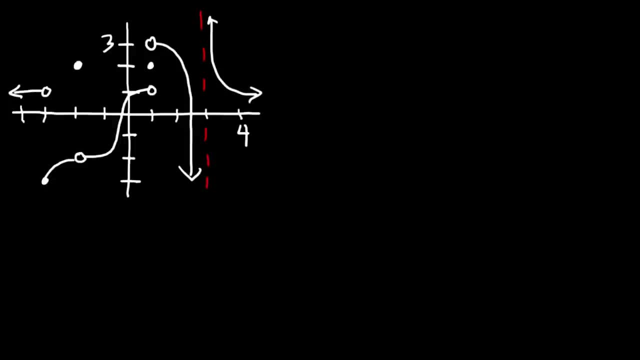 Now let's talk about how to evaluate limits graphically. So let's say, If we want to calculate the limit As x approaches negative 3 from the left side, And let's say this graph represents the function f of x. So what can we do? 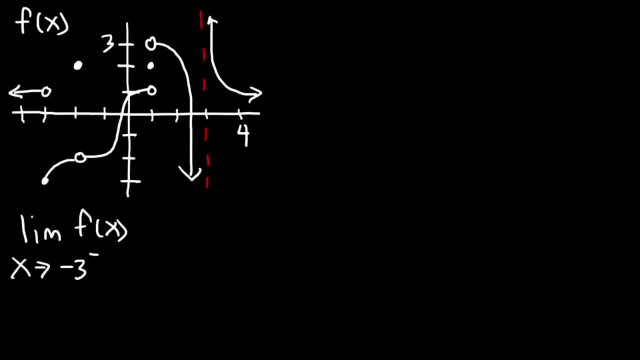 So to evaluate the limit you're looking for the y value. So first identify where x is negative 3.. x is negative 3 anywhere along that vertical line. Now we want to approach that vertical line from the left side. So therefore you want to follow the curve from the left until you get to that point. 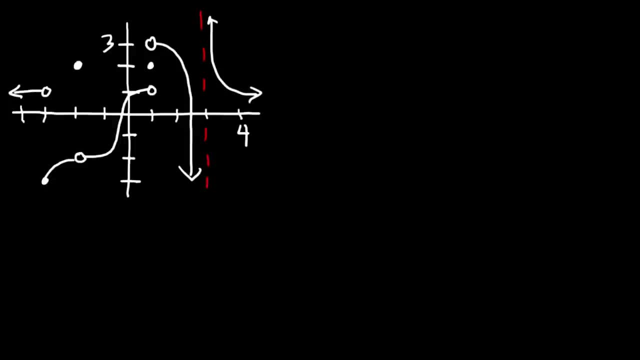 going to be the limit. Now let's talk about how to evaluate limits graphically. So let's say, if we want to calculate the limit as x approaches negative 3 from the left side, And let's say this graph represents the function f of x. 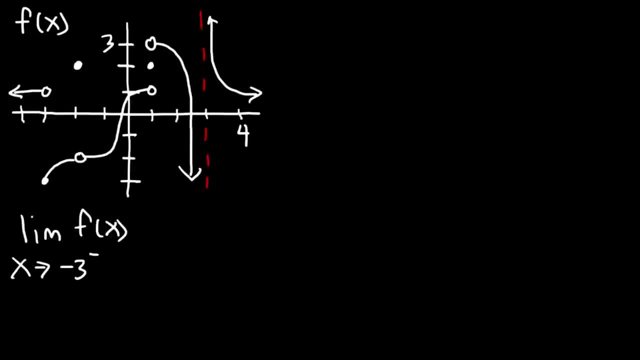 So what can we do? So to evaluate the limit? you're looking for the y value. So first identify where x is negative 3.. x is negative 3 anywhere along that vertical line. Now we want to approach that vertical line from the left side. 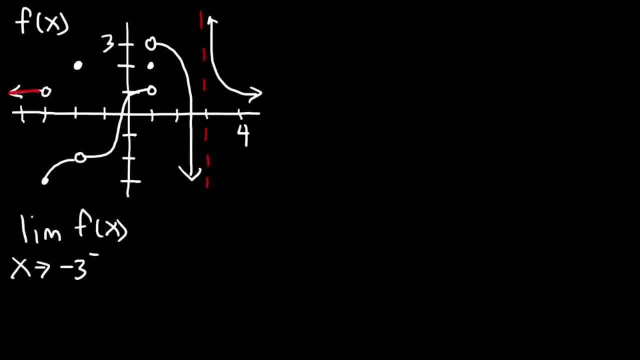 So, therefore, you want to follow the curve from the left until you get to that point. So notice that the y value here corresponds to positive 1.. So therefore, the limit as x approaches 3 from the left side is 1.. Now what about from the right side? So you want to approach the vertical line. 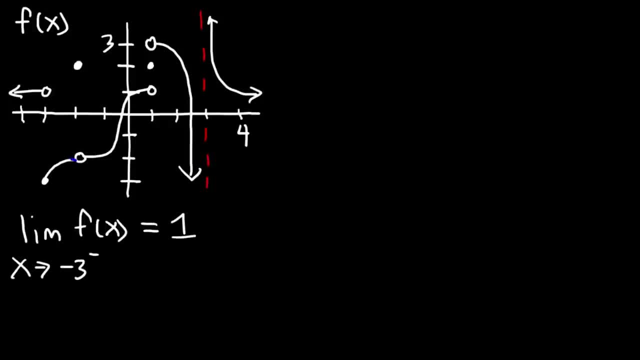 at negative 3 from the right. So we got to follow this curve. So notice that the y value here is negative 3.. So therefore the limit as x approaches negative 3 from the right side, that's negative 3.. Now what about? 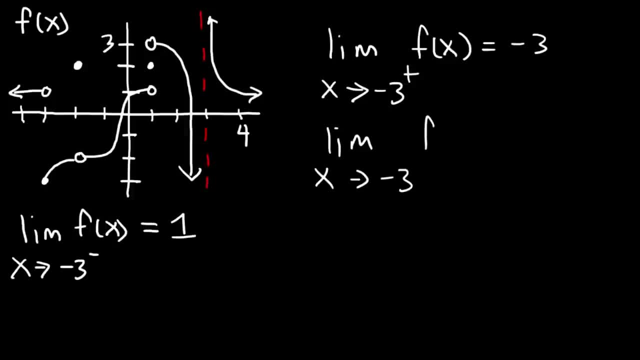 limit as X approaches negative 3 from either side. If the left-sided limit and the right-sided limit are not the same, then the limit does not exist. So these two are known as one-sided limits. Now what about F of negative 3? What is the? 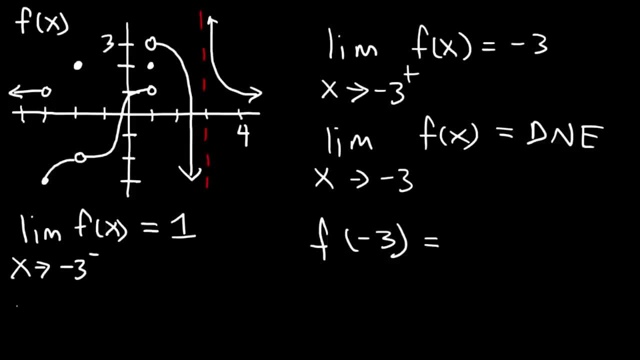 value of the function when X is negative 3? To find it, identify the closed circle which has a y-value of negative 3.. So this is it. Now let's work on some more problems. So what is the limit as X approaches? 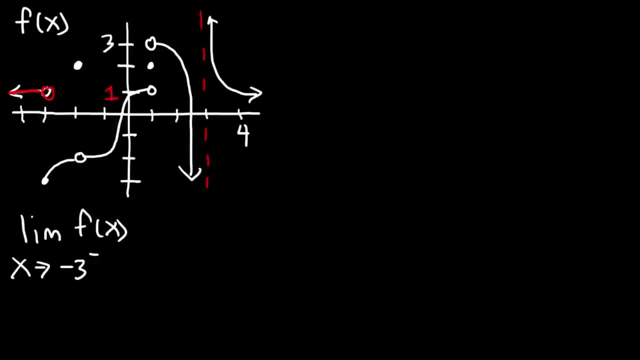 So notice that the y value here corresponds to positive 1.. So therefore, the limit as x approaches 3 from the left side is 1.. Now what about from the right side? So you want to approach the vertical line at negative 3 from the right. 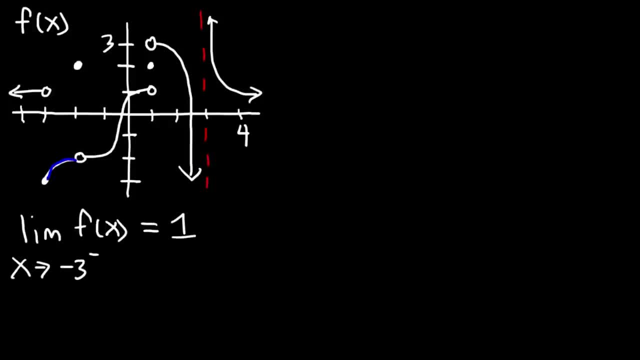 So we got to follow this curve. So notice that the y value here is negative 3.. So therefore, the limit as x approaches negative 3 from the right side, that's a negative 3.. Now what about the limit as x approaches negative 3 from either side? 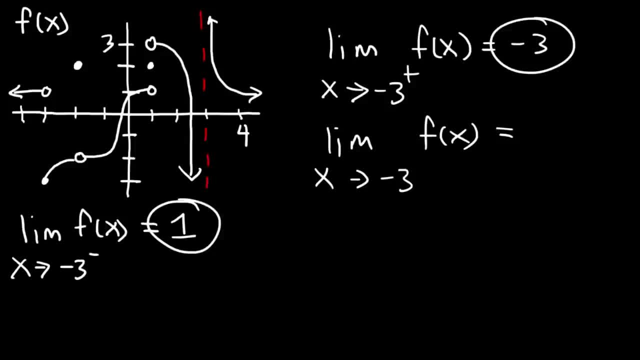 If the left sided limit and the right sided limit are not the same, then the limit does not exist. So these two are known as one sided limits. Now what about f of negative 3?? What is the value of the function when x is negative 3?? 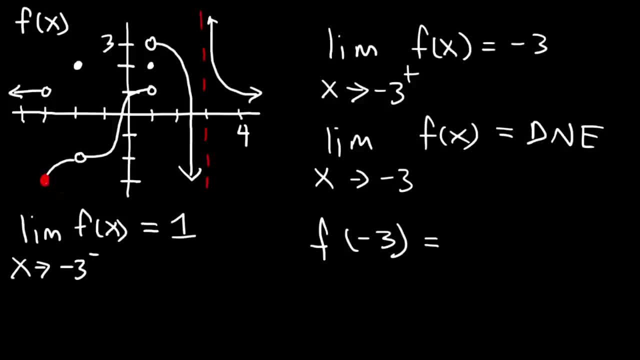 To find it, identify the closed circle which has a y value of negative 3.. So this is it. Now let's work on some more problems. So what is the limit as x approaches negative 2 from the left side? Go ahead and try this one. 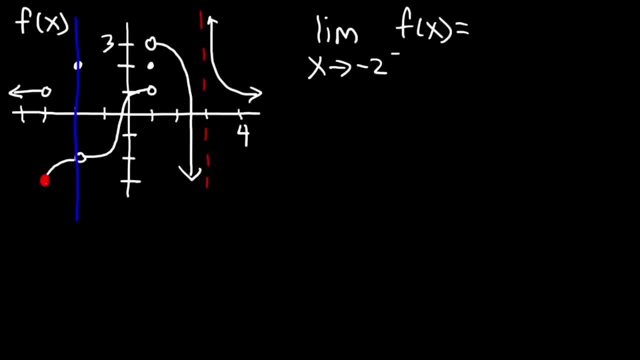 So identify the vertical line at negative 2.. So we want to approach that line from the left side. So what is the limit as x approaches negative 2 from the right side? So notice that the y value it negative 2.. So what is the limit as x approaches negative 2 from the right side? 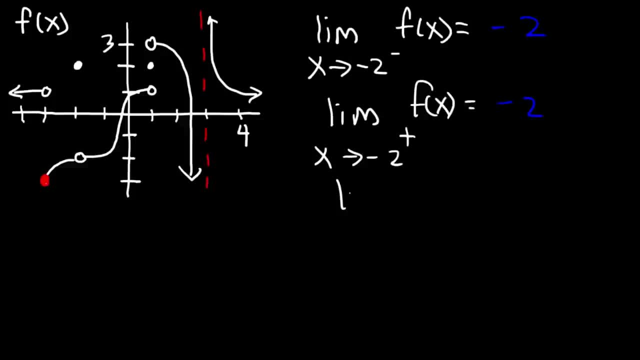 So this time we want to approach the vertical line from the right and it points to the same value: negative 2.. So notice that the y value is negative 2.. is negative 2 from either side does exist because these two, they match. 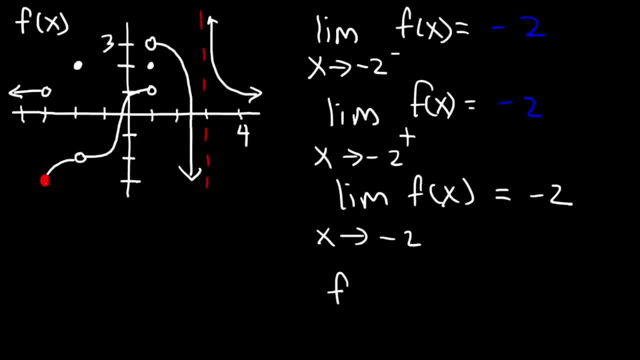 So therefore, it's going to be negative 2.. Now what is the function value when x is negative 2?? So look for the closed circle that's on this vertical line, And so that's this point where the y value is positive 2.. 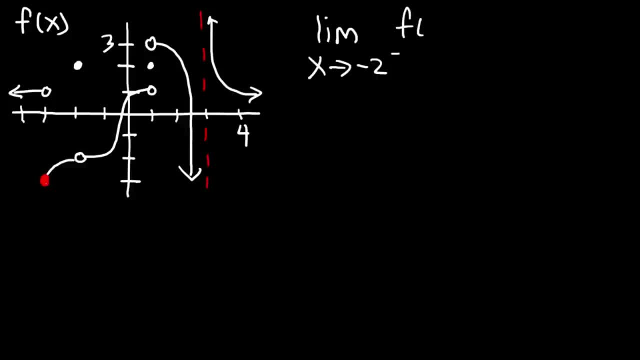 negative 2 from the left side. Go ahead and try this one. So identify the vertical line at negative 2.. So we want to approach that line from the left side. So notice that the y-value is negative 2.. So what is the? 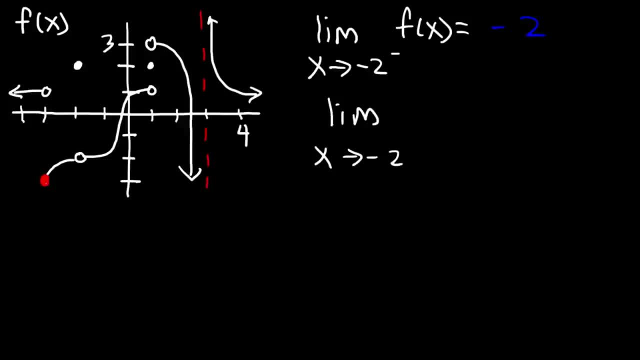 limit as X approaches negative 2 from the right side. So this time we want to approach the vertical line from the right, and it points to the same value, negative 2.. So therefore, the limit as X approaches negative 2 from either side does exist. 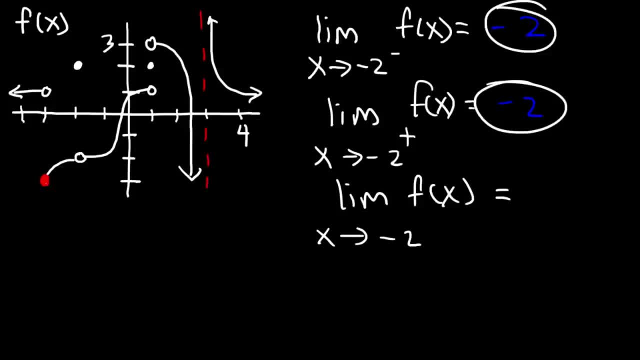 because these two match. so therefore it's going to be negative 2.. Now what is the function value when X is negative 2?? So look for the closed circle that's on this vertical line, And so that's this point where the y-value is positive 2.. So 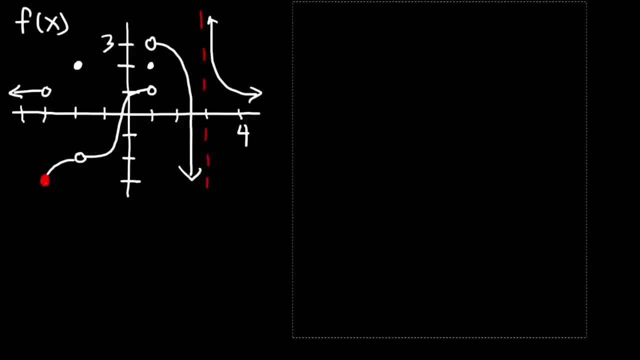 So, as you can see, it's not very difficult to evaluate limits graphically. Now let me give you a new set of problems. Evaluate the limit as X approaches positive 1 from the left side, from the right side and from either side. 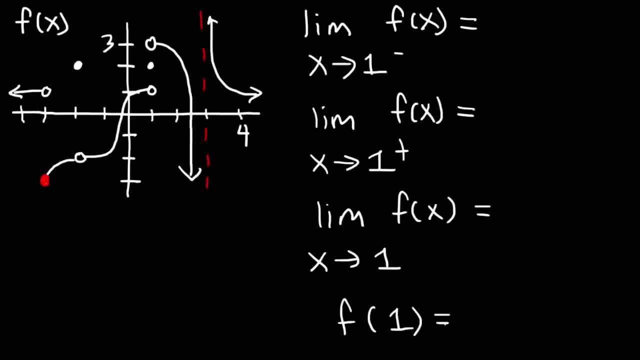 And also find the function value when X is 1.. So X is 1 anywhere along that vertical line. So if we approach it from the left side, notice that the Y value is positive 1 there, And if we approach it from the right side, the Y value is 3.. 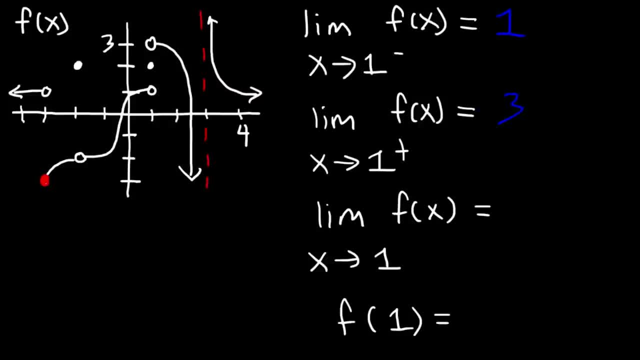 So, because these two do not match The limit, as X approaches, positive 1 from the right side is positive 1.. As X approaches, 1 does not exist. Now the function value at 1 is the closed circle, which has a Y value of 2.. 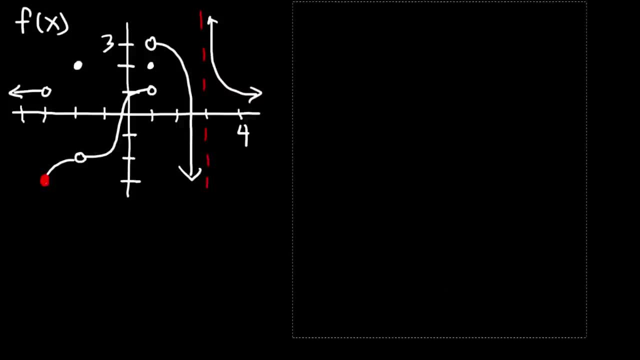 So, as you can see, it's not very difficult to evaluate limits graphically. Now let me give you a new set of problems. Evaluate the limit as x approaches positive 1 from the left side, from the right side and from either side. 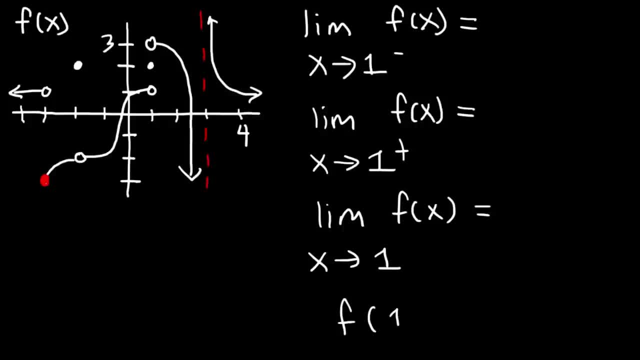 And also find the function value when x is 1.. So x is 1 anywhere along that vertical line. So if we approach it from the left side, notice that the y value is positive 1 there, And if we approach it from the right side, the y value is 3.. 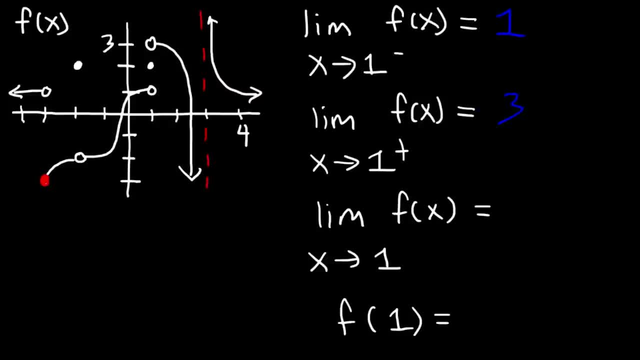 So, because these two do not match the limit, as x approaches, 1 does not exist. Now the function value at 1 is the closed circle which has a y value of 2.. Now here's the last set of problems like this: 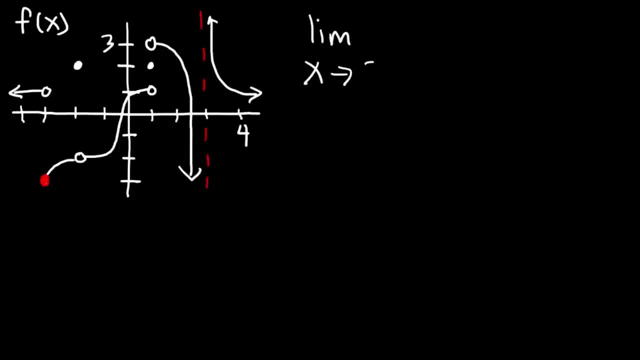 What is the limit? as x approaches positive 3 from the left side and from the right side, So x approaches positive 2 from the left side and from the right side, and from the right side and from the right side. Okay, 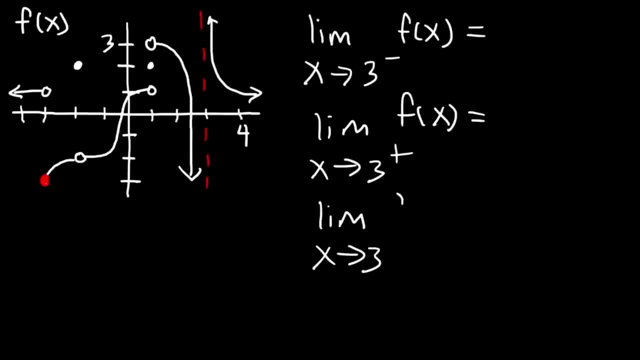 and from either side, and then find the function value at 3.. So notice that at x equals 3, we have this vertical asymptote. So as x approaches 3 from the left side, notice that it goes down to negative infinity. 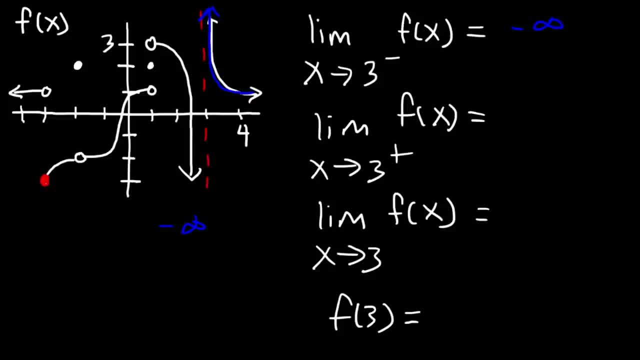 And as we approach 3 from the right side, it goes all the way up to positive infinity. Now these two do not match, so therefore the limit does not exist And the function value at 3 is going to be undefined. 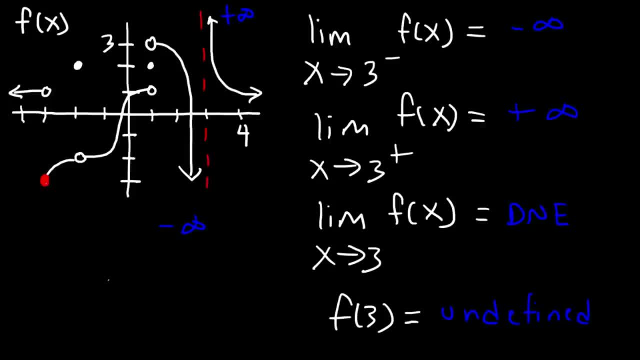 So a good example of having a vertical asymptote at x equals 3 would be a function like this: 1 over x minus 3.. And if you plug in 3, you're going to get 1 over 0, which is undefined.